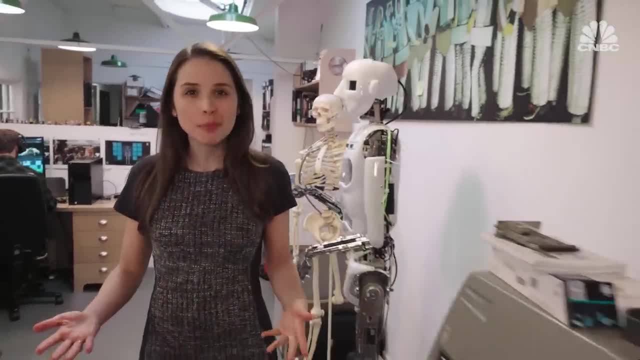 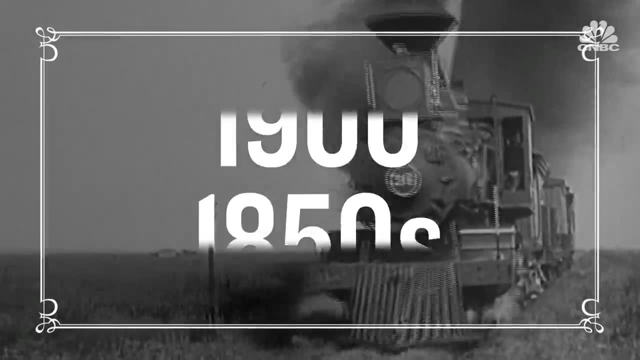 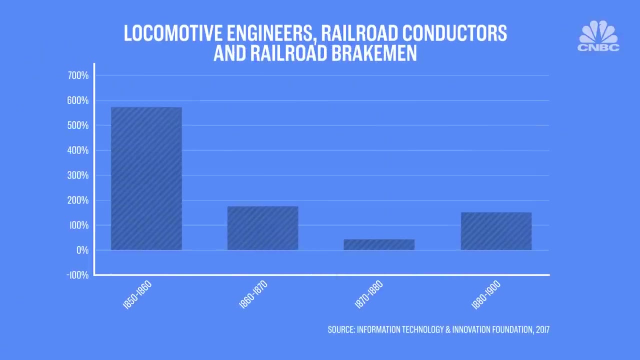 Many economists argue automation will ultimately create new jobs. After all, someone has to program the robots right. Let's go back to the 1850s, when trains were the most popular mode of transportation. This chart shows the number of locomotive engineers, railroad conductors and brakemen increasing by nearly 600%. 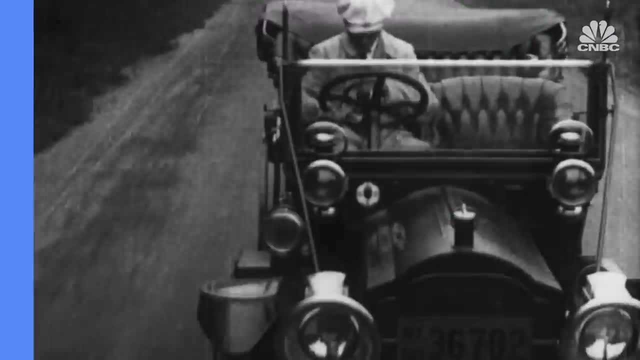 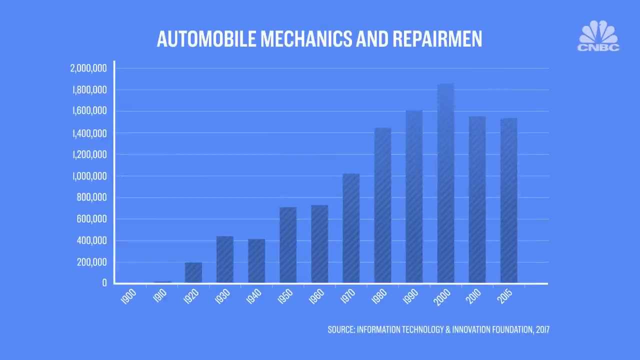 But that growth slowed in the early 1900s. Why? You guessed it? The automobile came along. Car mechanic and repairman jobs surged, even though railroad jobs began to disappear, And some companies say the same thing will happen when robots move into the marketplace. 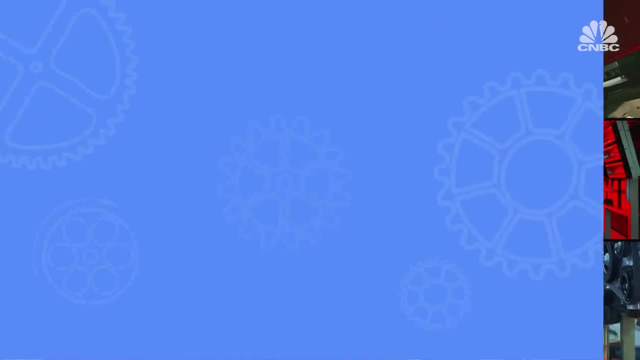 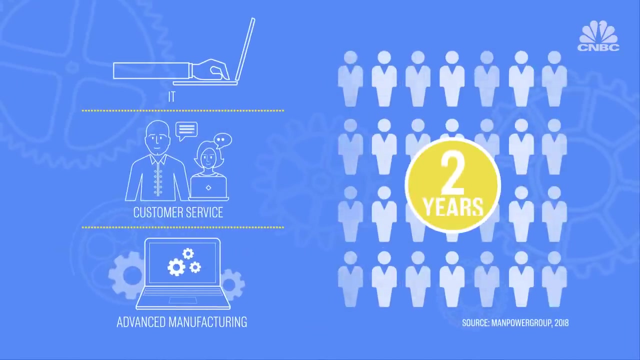 A survey of 20,000 employers from 42 countries found that the IT, customer service and advanced manufacturing industries will add workers over the next two years as a result of automation. It's hard to imagine that robots could replicate human characteristics like empathy or compassion. 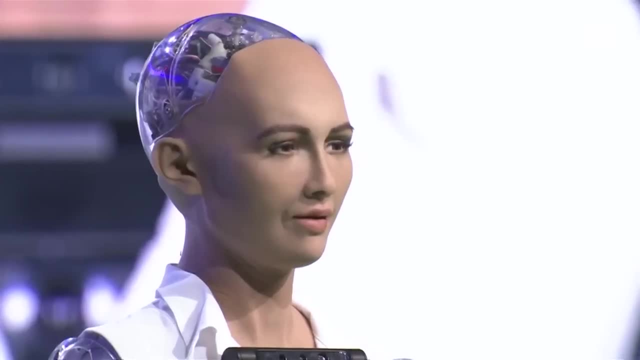 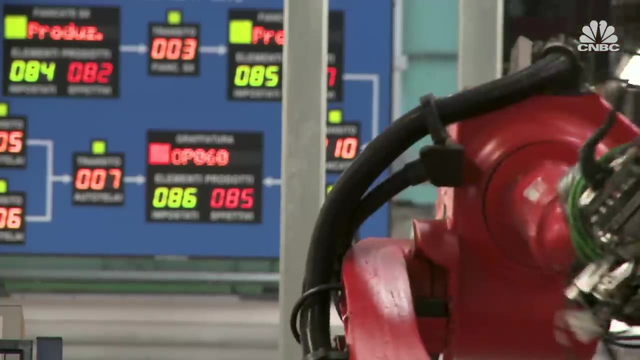 that are required in many jobs. I mean, would you really want a robot as your nurse, babysitter or teacher? But even if robots don't take our jobs entirely, research shows they will significantly change day-to-day tasks in the workplace. 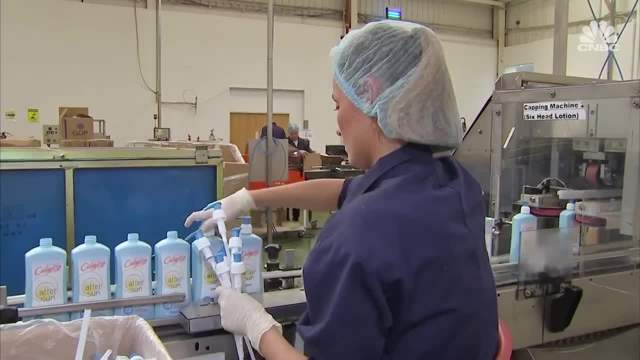 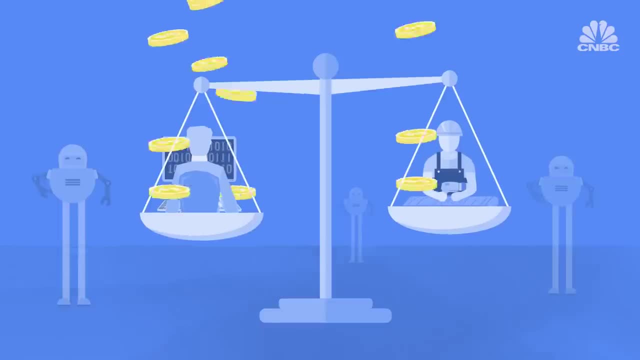 This is particularly a problem for lower-skilled workers who aren't able to retrain for new jobs. They might get stuck with lower wages in a world with more robots, and that could make income inequality even worse. These guys are making a lot of things uncertain right now. 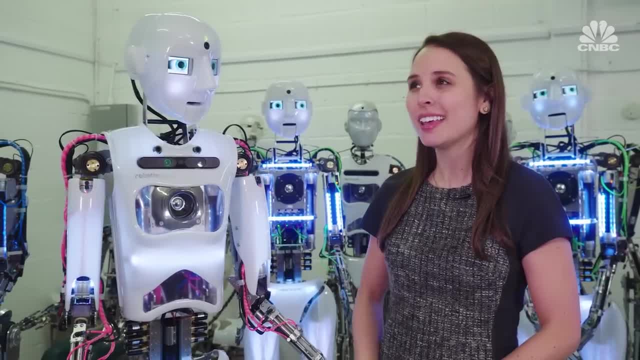 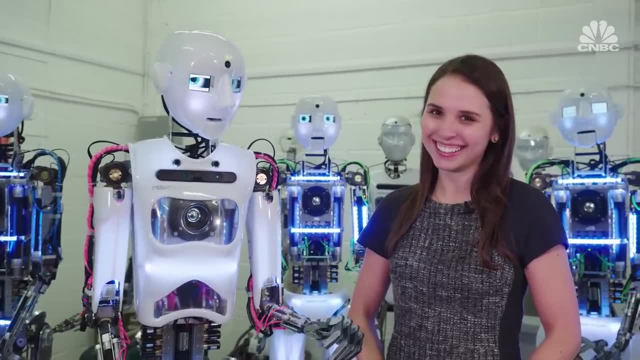 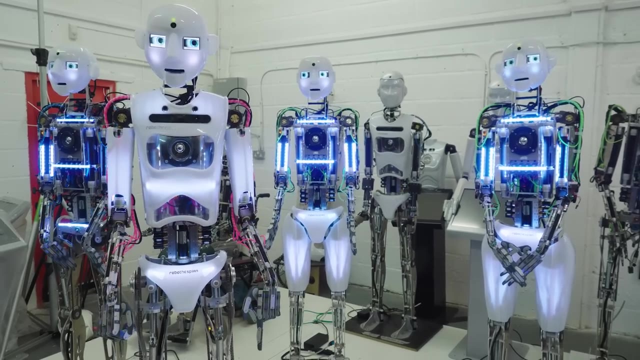 But one thing that's clear is: skills training is required if we hope to get along with friends like them in the workplace. I think we're going to get along just fine. Hey everyone, it's Elizabeth and RoboSaskian here. Thanks so much for watching our video. 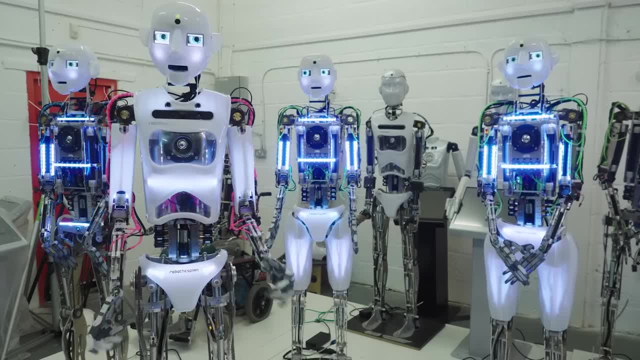 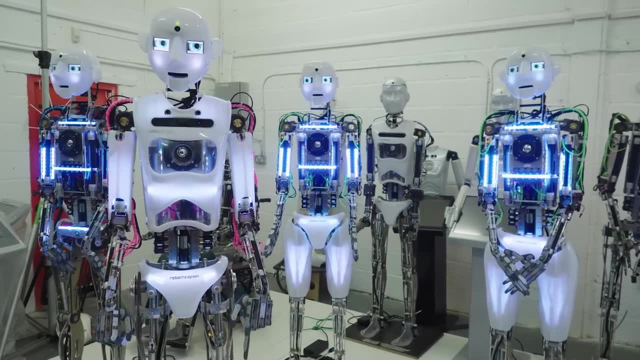 You can check out more of our videos all the time, including one about universal basic income, over here on our YouTube page. While you're at it, leave us some ideas in the comment section and subscribe to our channel. See you later. Subtitles by the Amaraorg community.